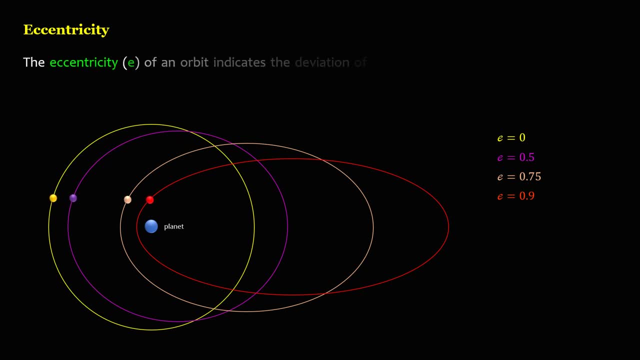 The excentricity e- of an orbit indicates the deviation of the orbit from a perfect circle. A circular orbit has an eccentricity of zero, while a highly eccentric orbit is closer to, but always less than one. A satellite in an eccentric orbit moves around one of the ellipses' focal points, not the center. 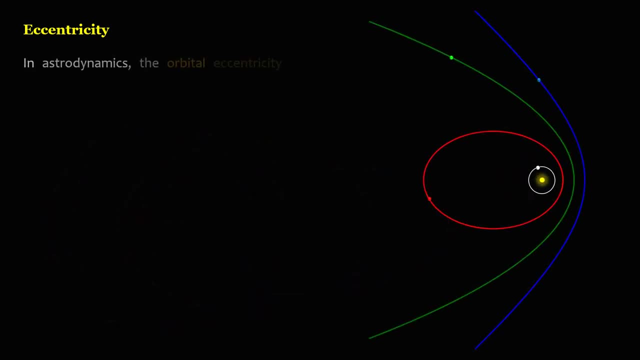 RX. In astrodynamics, the orbital eccentricity of an astronomical object is a dimension, dimensionless parameter that determines the amount by which its orbit around another body deviates from a perfect circle. A value of zero is a circular orbit. Values between zero and one form an elliptic orbit, One is a parabolic. 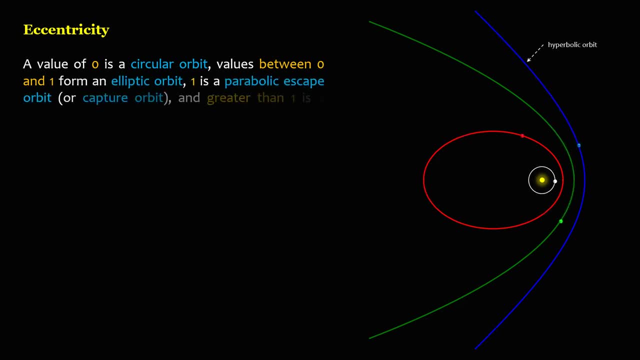 escape orbit or capture orbit and greater than one, is a hyperbola. The eccentricity E may take the following values: Circular orbit E equals zero. Elliptic orbit E greater than zero. less than one Parabolic trajectory E equals: 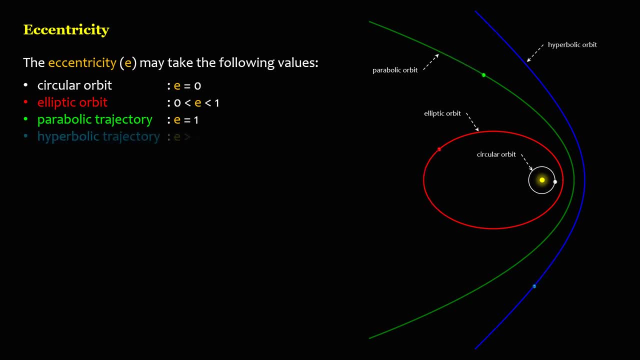 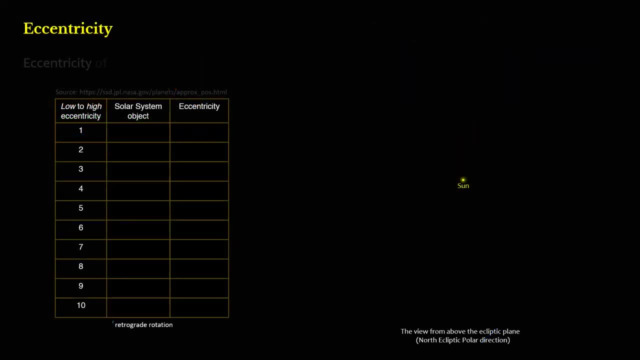 one Hyperbolic trajectory E greater than one Eccentricity of the inner planets and Jupiter, Mercury, Venus, Earth, Mars, Jupiter. Eccentricity of the gas and ice giants, Pluto and Halley's Comet, Jupiter. 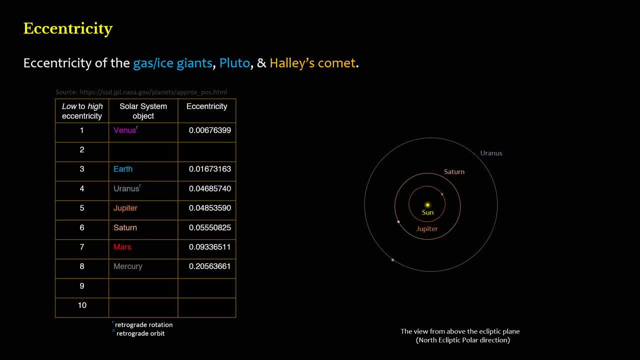 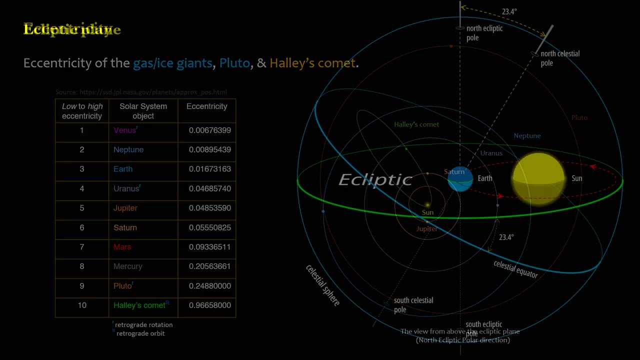 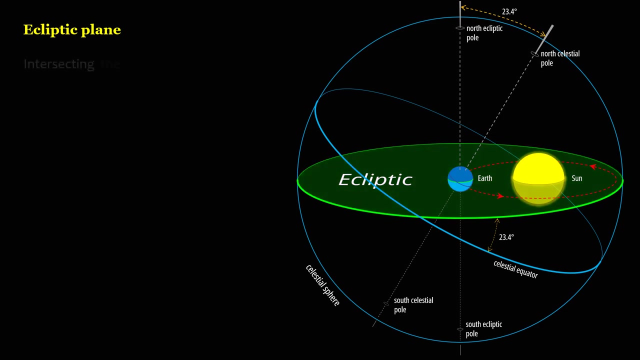 Venus, Saturn, Uranus, Neptune, Pluto, Halley's Comet, Eurasians, Atom altar or planet. The ecliptic is the plane of Earth's orbit around the Sun. Intersecting the celestial sphere is the ecliptic plane. This is the plane in which the planets and Bogus are in contact with. The warmed airretие of the general himself is a verticalалась of X-ray and basement body. This is the plane in which the parameters of Jupiter don't necessarily need to belong here or beyond either objects, So one'sED comes from either person. tovär, diesel, atom devegates, male or female, energy commissions, Deeper universes, All barabia and German.